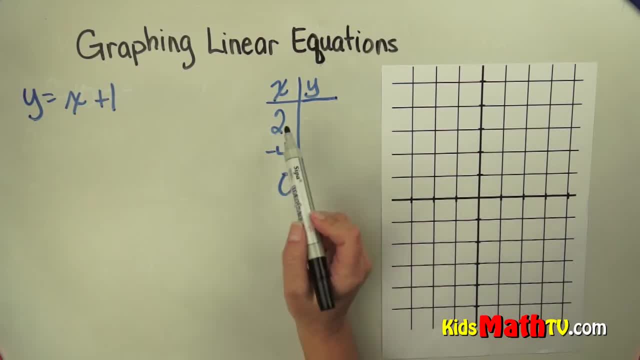 some basic, simple numbers. So now what I'll do is I will substitute this x value into this equation, So y equals x, which is now 2, plus 1.. And when I solve that, y equals 3.. So with this equation, if x is 2, y is 3.. So let's try it again: Y equals x plus 1.. 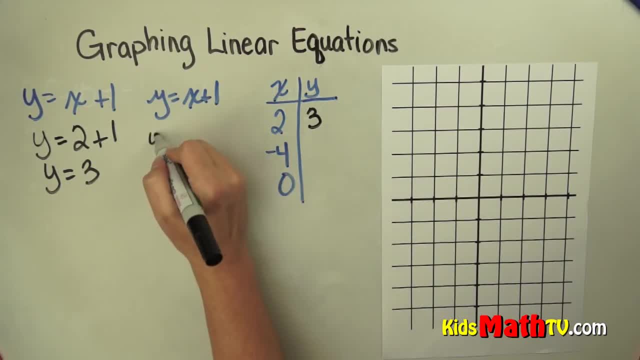 This time we will use the value negative. 4 for x- Y equals negative 4 plus 1.. Ok, Ok, Ok, And if I add negative 4 to 1, I get negative 3.. So if I have negative 4, as my x- y is negative 3.. 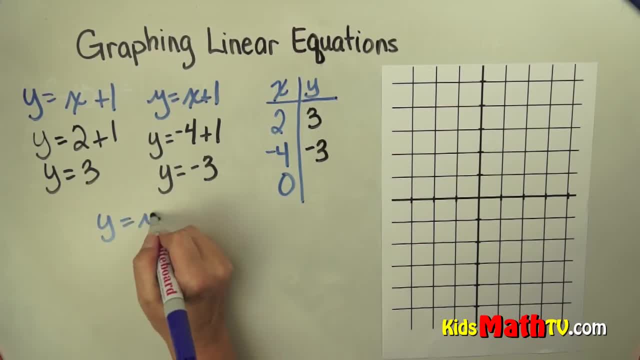 Let's try one more with 0.. y equals x plus 1.. I'm using the same equation. Substitute 0.. y equals 0 plus 1.. And y, let's see, 0 plus 1 is simply 1.. 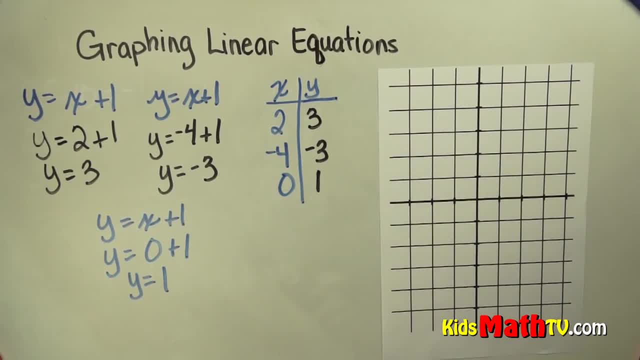 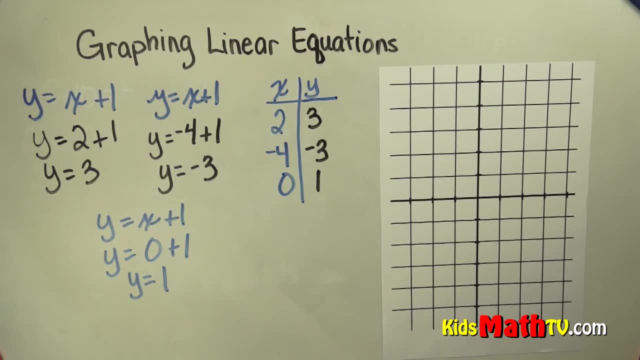 All right, so I'll do that in black so you can see it easily. Now I can graph these values on my coordinate grid. So 2, a positive 2 means I go to the right 2 times, And positive 3 means I go up 3 times. 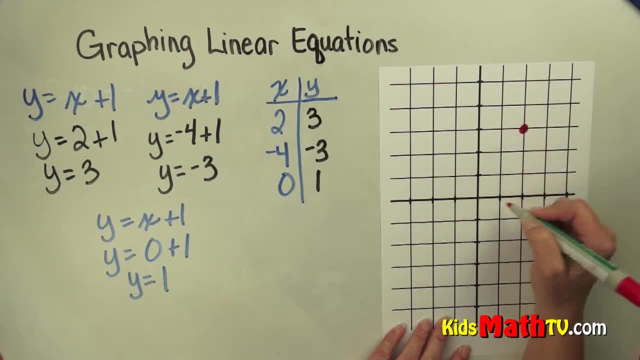 1,, 2, 3.. So that is positive 2, positive 3.. Then I have negative 4, negative 3.. Negative 4 means I go to the left 4.. 1,, 2, 3.. 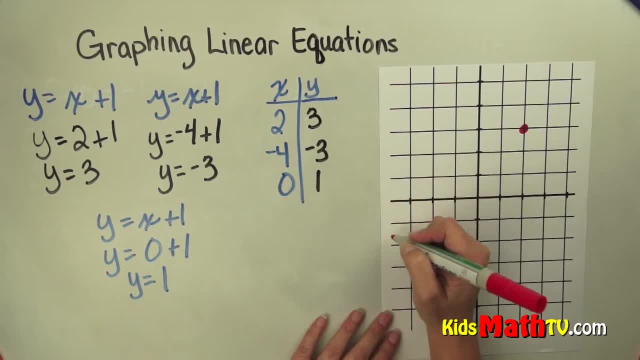 4. And down 3, because it's a negative 1,, 2,, 3. And 0 means that I don't move on the x-axis. Positive 1 means I go up 1. So 0, positive 1.. 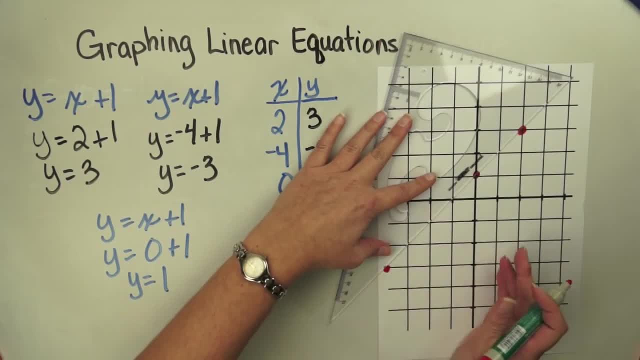 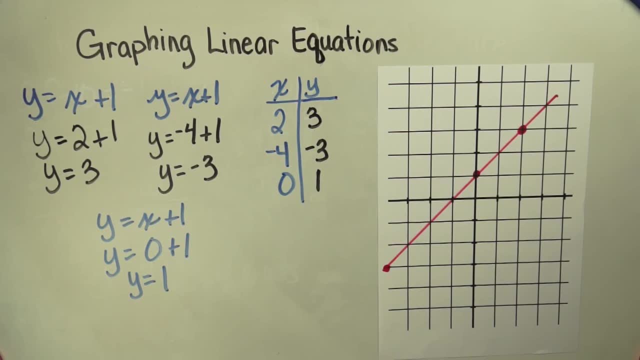 And then I take my straight edge and line up those points And there is the line, And that's the end of this lesson on graphing linear equations. Thank you, Thank you.